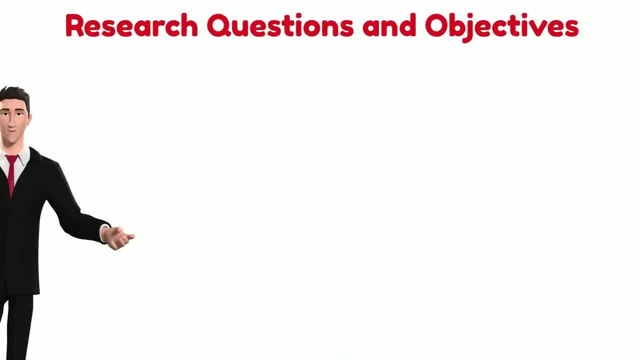 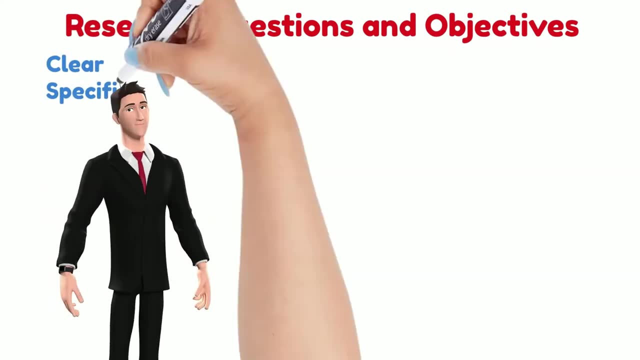 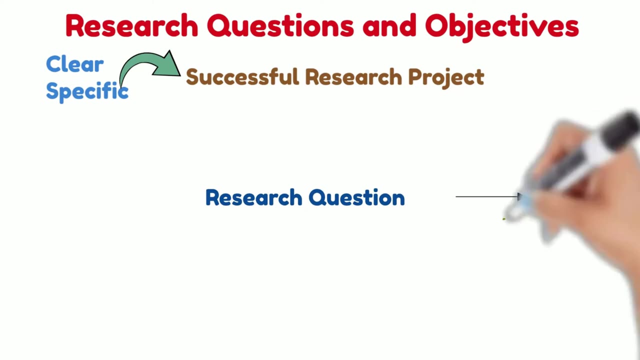 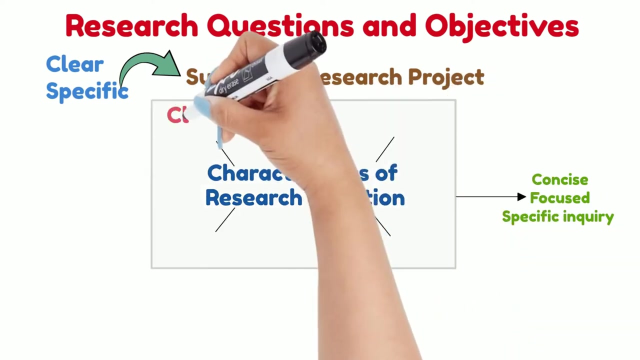 Research questions and objectives provide direction and purpose for a research study. Clear and specific research questions and objectives are essential for a successful research project. A research question is a concise, focused and specific inquiry that guides the research process. Characteristics of a good research question include being clear. 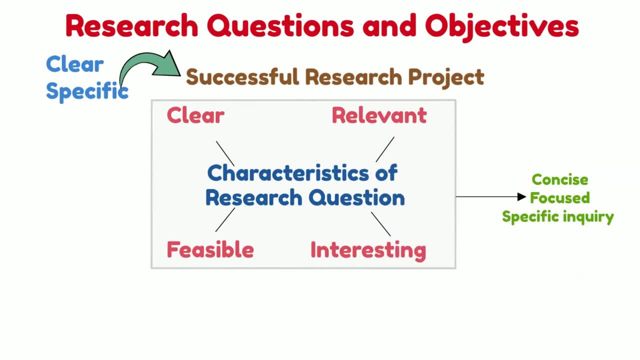 relevant, feasible and interesting. These are examples of research questions. What are the effects of social media on mental health among adolescents? How do changes in temperature affect the growth of bacteria? What is the relationship between job satisfaction and turnover among healthcare workers? Research objectives are specific. 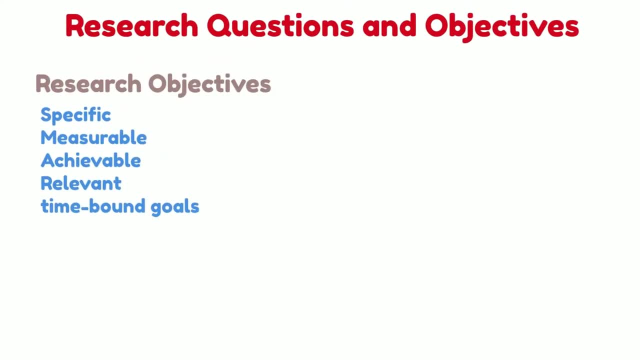 measurable, achievable, relevant and time-bound goals that guide the research process. Good research objectives provide direction and focus for the study and help to ensure that the study is feasible and achievable. This is the example of research objectives To determine the effectiveness of a mindfulness-based stress reduction program. 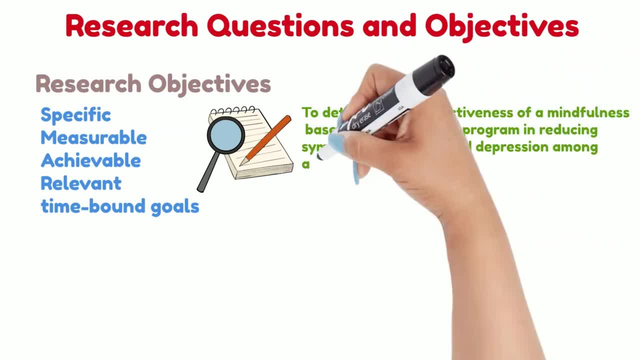 in reducing symptoms of anxiety and depression among adults with generalized anxiety disorder. This research objective is specific, measurable, achievable, relevant and time-bound. It identifies the target population: adults with generalized anxiety disorder. the intervention being studied: a mindfulness-based stress reduction program. 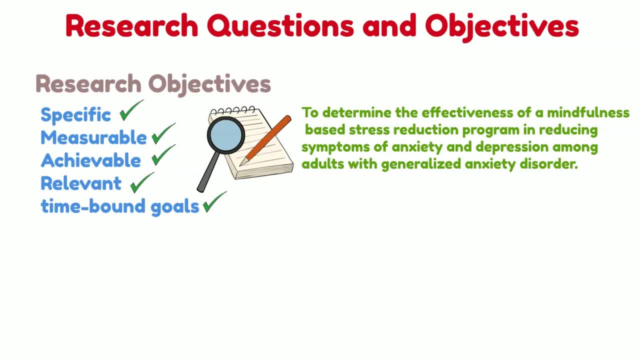 and the outcome being measured- reduction in symptoms of anxiety and depression. The objective is feasible and relevant to the research problem being addressed, and it has a clear timeline for completion. Research questions and objectives should be aligned with the research design in order to ensure that the study is feasible, relevant and time-bound. To determine the effectiveness of a mindfulness-based stress reduction program in reducing symptoms of anxiety and depression among adults with generalized anxiety disorder. it is necessary to determine the effectiveness of a mindfulness-based stress reduction program in order to ensure that the study is feasible, relevant and time-bound. 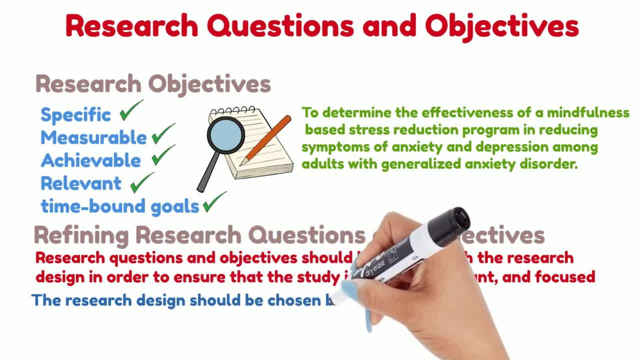 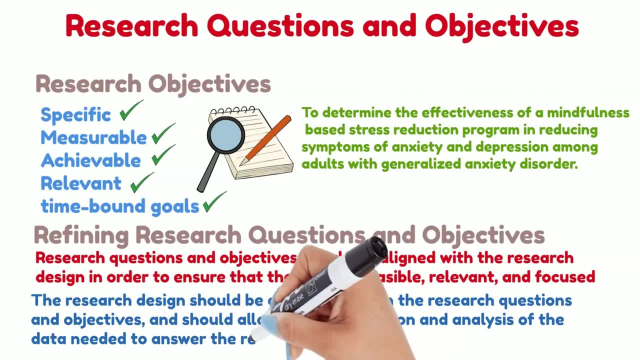 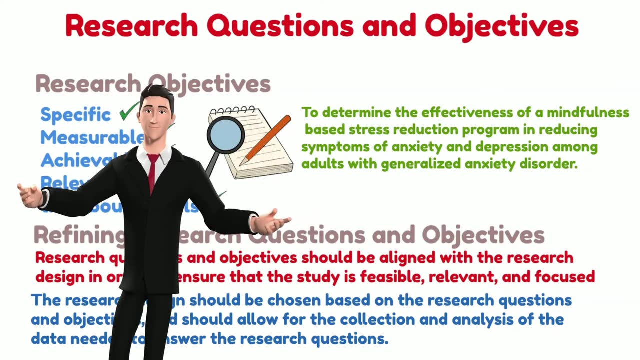 The research design should be chosen based on the research questions and objectives and should allow for the collection and analysis of the data needed to answer the research questions. Example: If the research question is: What are the effects of social media on mental health among adolescents?